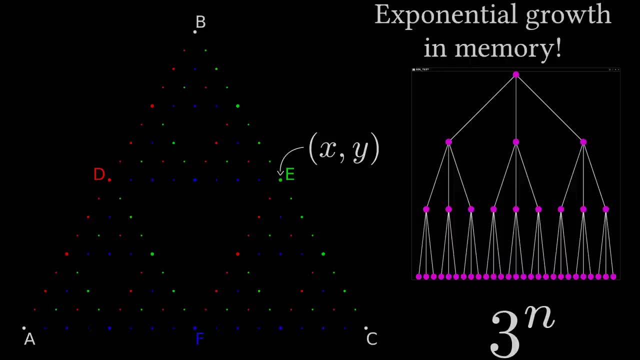 footprint also grows exponentially. Honestly, the simplest way of creating this animation would be to fully generate the tree we want in the end- in this case, up to four generations- and then do a breadth-first search over the elements. Now look, This would definitely work for the purposes of the video we were making at the time. We only 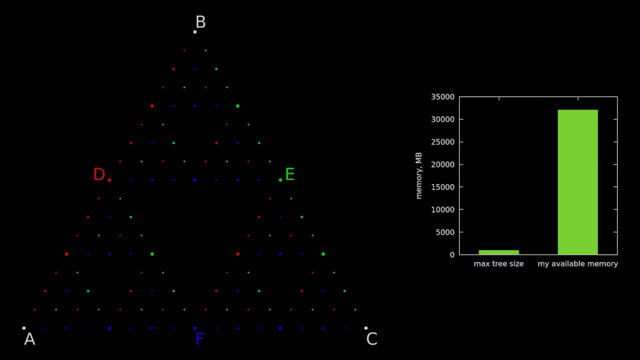 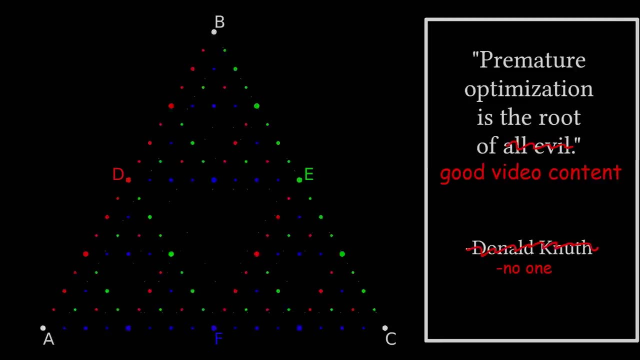 needed ten generations at most, so there was no reason not to store the entire tree in memory. But you know what they say: Premature optimization is the root of good video content. So what would we need to do if we wanted the largest possible Sierpinski triangle animation ever? 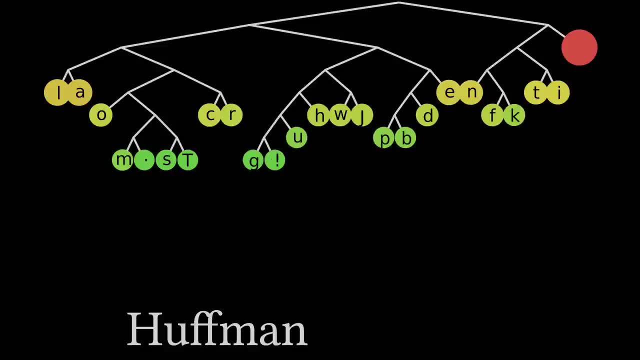 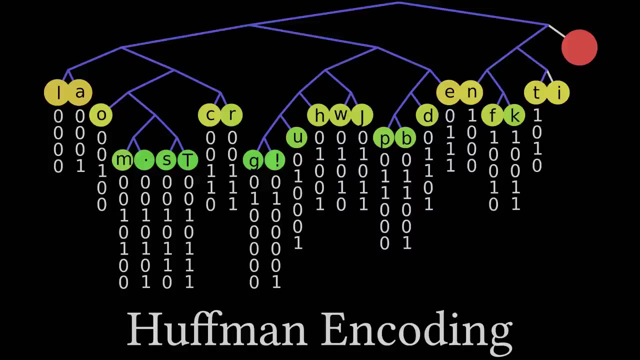 Well, let's go back to another fun topic: Huffman encoding. Here we were able to uniquely create a code word for each character in a string we wanted to encode by traversing through a tree. Every time we would go down the left branch, we would add a 0, and when we went down the right branch, we would add. 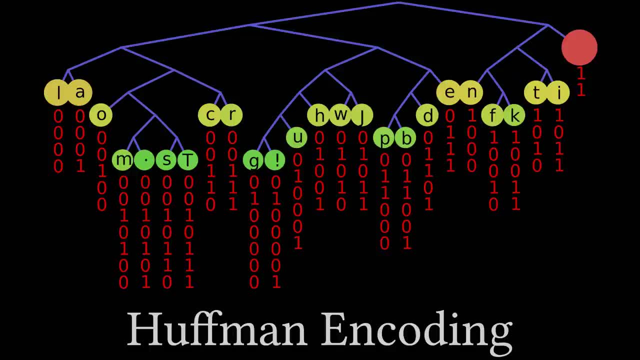 a 1.. What if the final string of 1s and 0s was actually a set of functions to apply? That is to say, the string 0, 1, 0 would mean applying function 0,, function 1, and then. 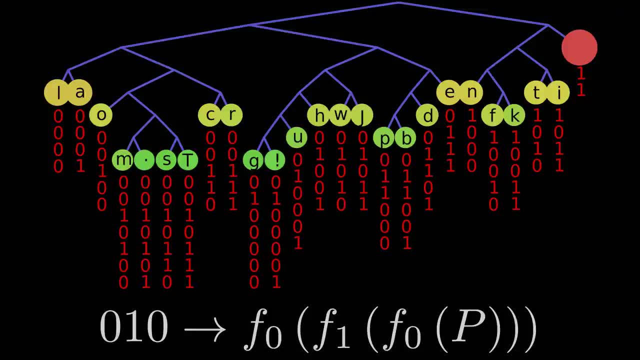 function 0 again to our root node's location. In that case, each node would no longer need to keep a location, but instead a set of functions. In this case, each node would no longer need to keep a location, but instead a set of functions. 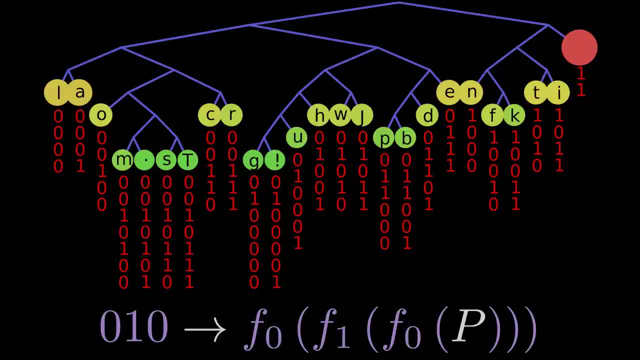 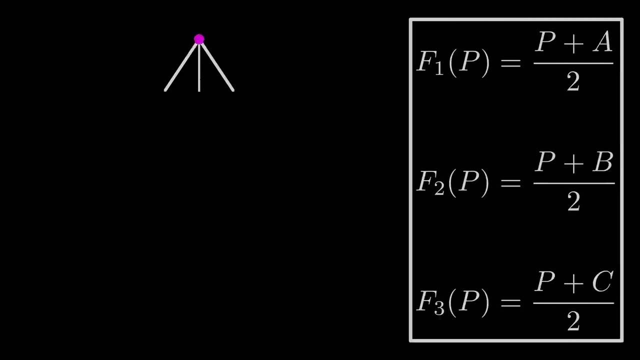 This is a bit more than that, because we have a set of 3 functions for this animation, we couldn't really use traditional bit, but would instead need to use base 3 bits, sometimes called trit's in a bijective 3-based number system. This simply means that our 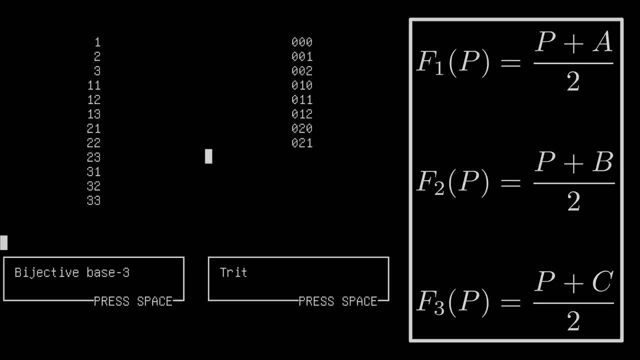 counting would need to look like this and not like this. In some sense, this directly solves our memory issue. Essentially, a breadth-first search for this might not quite deliver the exact same performance as JUST1, but we'll find some more ways to do this. 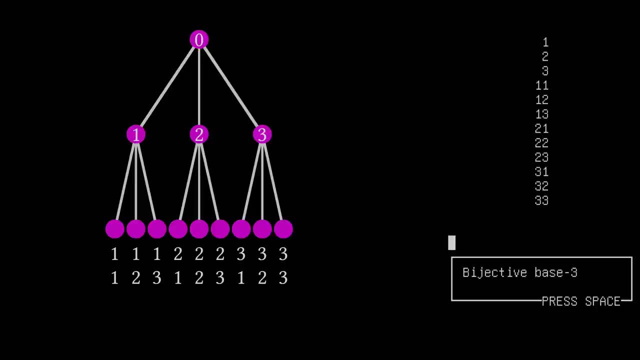 tree is actually just counting in bijective base three trit space. This means that instead of having to keep an entire tree in memory, we just need to keep a trit string and increment it by one each time. After that, we can interpret each trit string as a series of functions to implement.